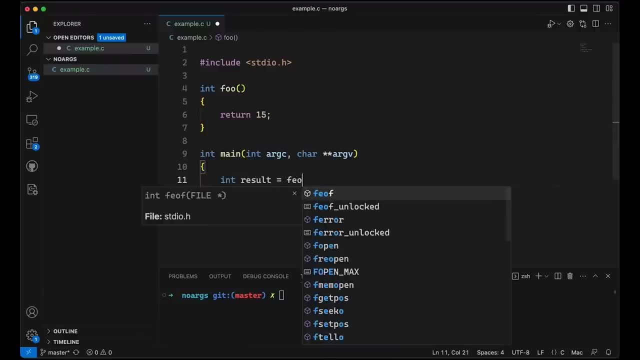 here. let's just say int result Equals foo, And then I'm going to printf: result is percent D And then we'll print out result. Okay, so pretty simple. I shouldn't create a make file. That's really unusual for me. 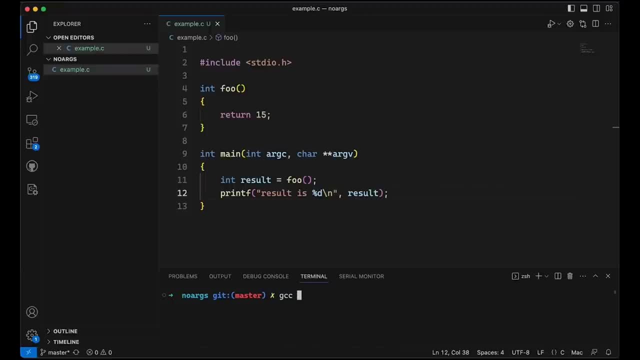 but that's okay. So let's just come down here and we will do gcc, dash g example, dot c example, And so I can compile it. Great, no problem, And we can run example, right. So it worked fine. It worked the way we expected. Really no worries. Now what if I later on came? 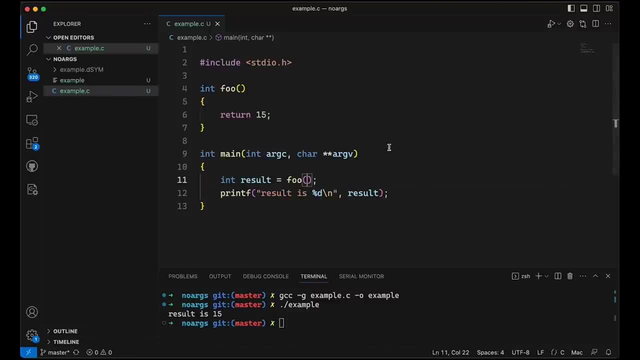 down here and let's say I'm changing some things around and I accidentally add a bug to my code and I say something like I add a 12 here, thinking hey, I'm going to pass an argument to this, even though up here it doesn't take an argument. But so if I do this and I come back, 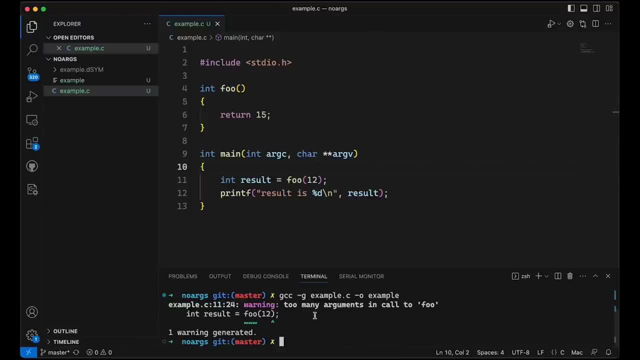 down here and I go to compile it. So here I'm going to get a warning which is really useful. Now, I mean, because I passed too many arguments to it. Let's just make sure that clang does this as well. Yeah, so they're both giving me a warning, And then I'm going to go ahead and 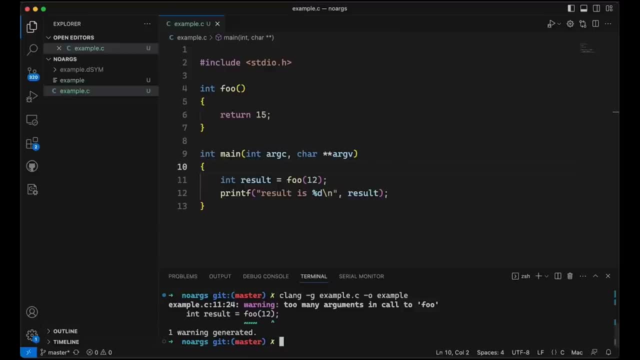 these warnings saying, hey, this might not be what you want to do, But it's interesting that this is a warning. you know, it's a warning meaning my code still compiled, I can still come in here and say example, and it still runs. So the question is, why didn't this give me an 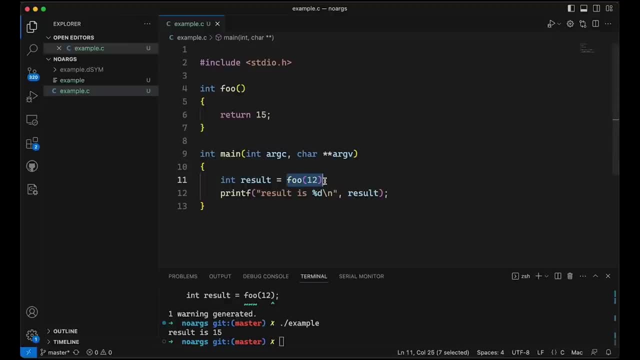 error. right, I called this function incorrectly, right? Well, actually that's not the case According to the C language. when you don't put anything in here, that just means this function can take zero or more arguments. If I wanted to tell the compiler that this must always. 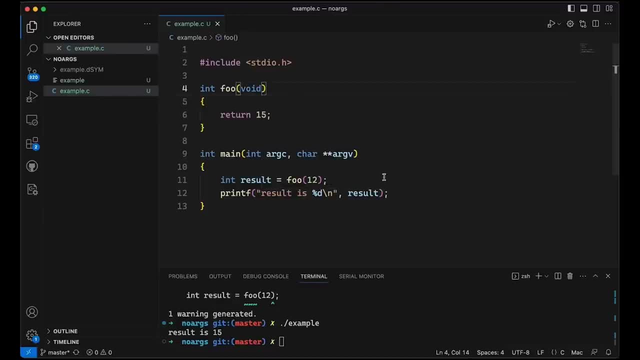 have no arguments, I should say: void here. Okay, now let's see what happens. Let's see how this looks different Now if I come in here and I compile. well, if you come in here now, we get an. 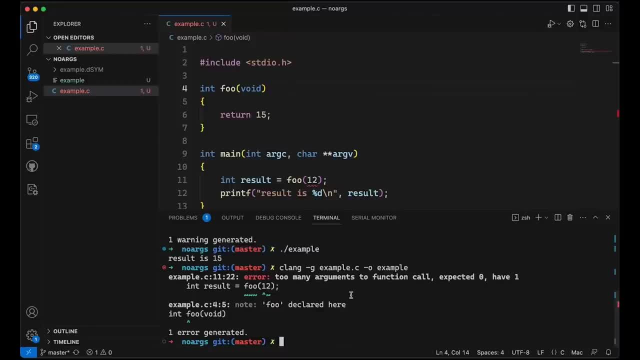 error. right Now it actually enforces this and says: now I'm not going to compile this, because you said that it takes no arguments up here, and then you use it with an argument, And so I'm not just going to throw a warning, I'm going to give you an error and this is not going to compile. 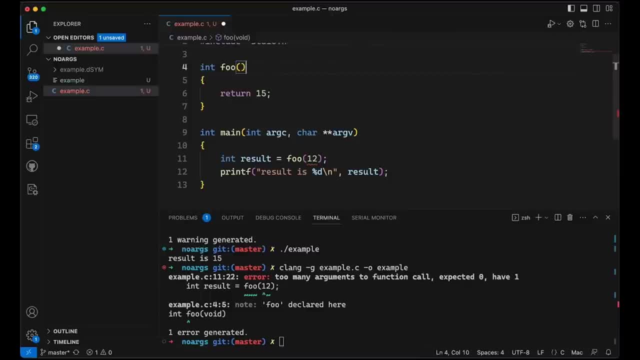 And in some older compilers there were times where you wouldn't even get a warning. it would just just compile and you just would kind of not give you what you wanted. maybe give some confusion, But you know it is in this case.